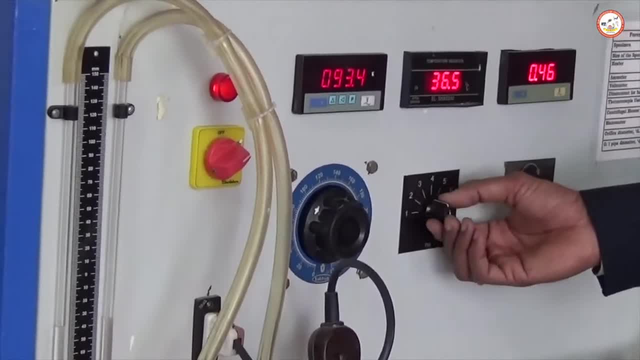 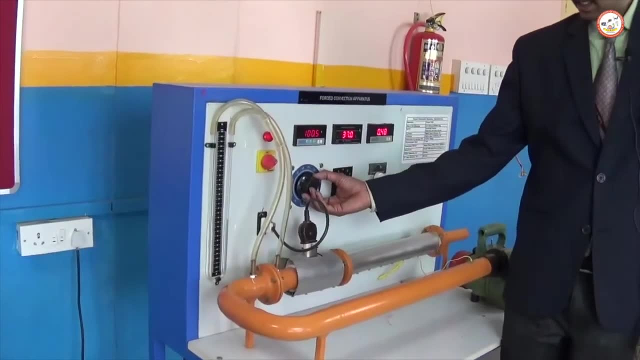 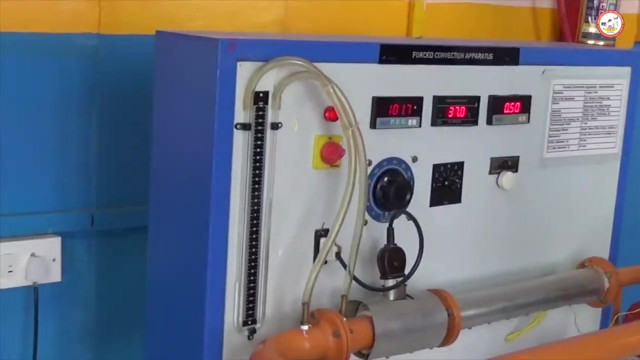 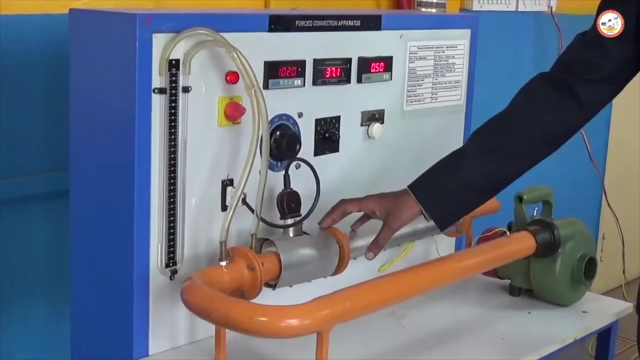 knob, And here, initially we have to switch on the operators and then you have to set the heater coil around 100.. Afterwards you have to switch on the blowers. As we switch on the blowers, the specimen through the U-shaped tube and you are going to supply the heat here Afterwards. 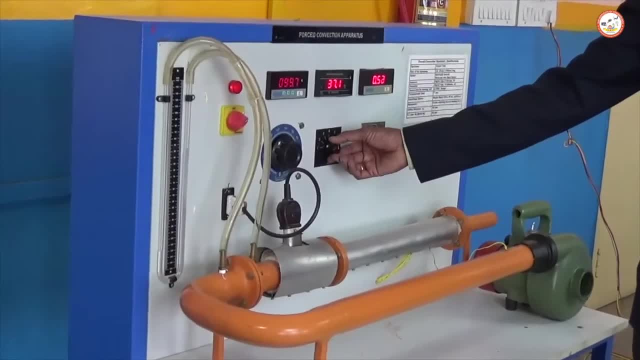 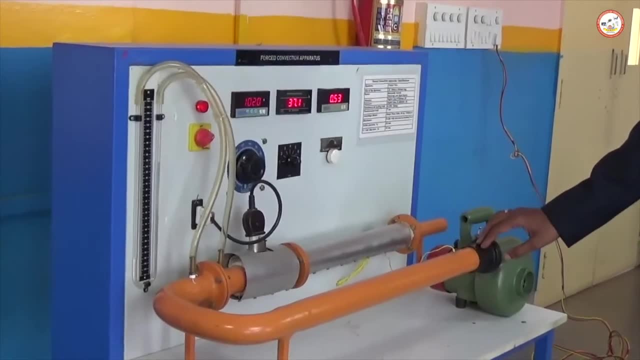 you have to note down the readings of the surface temperature: T1, T2,, T3,, T4 and T5. At the temperatures, after some time it will be come to the steady state. The repeated reading will be come to the same values. In that condition the experimental setup is on the steady state. 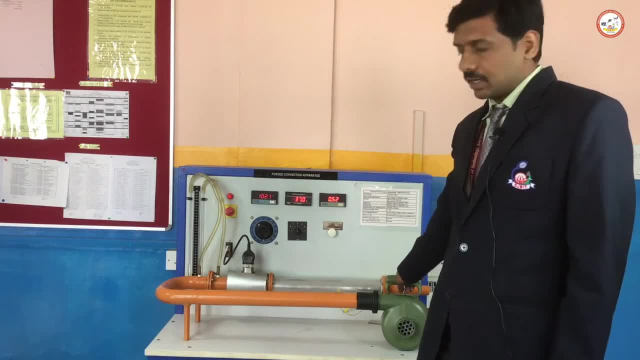 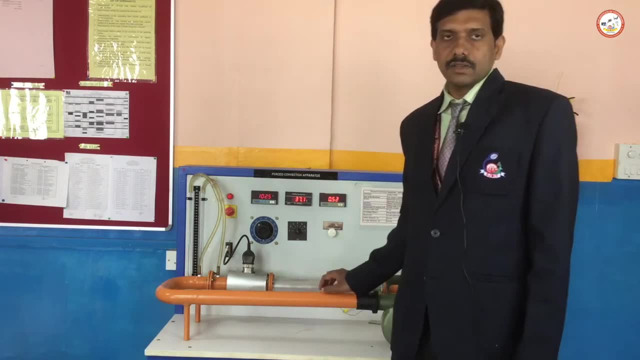 condition. At that time you have to note down all the readings and you have to do the calculations by using the equations. Q is equal to HA delta T, That is the connective heat transfer equations, And Q is the amount of heat supplied to the specimen by using the voltmeter and the ammeter. 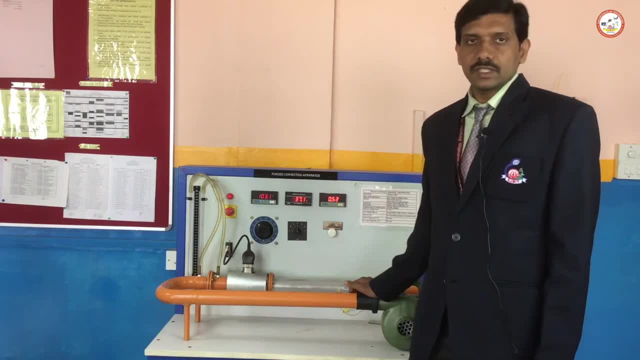 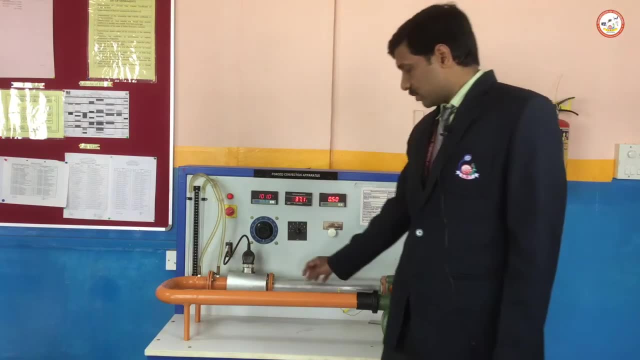 reading. Q is equal to V into 5. That will give the supply of the heat. And H is the heat transfer coefficient, That one you have to find out here. And A is the surface area of the specimen. Here the specimen is there On the surface. we are going to use the various thermocouples There. 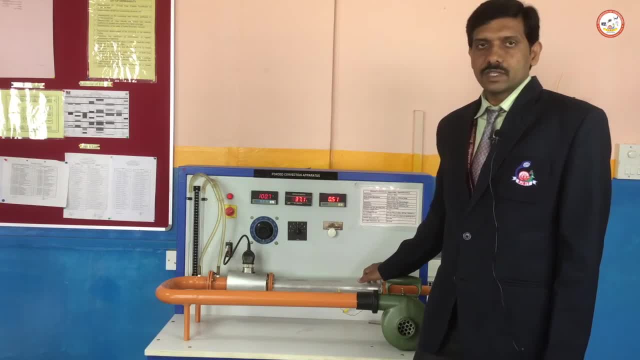 is nothing but the 5DL. that will give the surface area of the specimen And delta T is the temperature difference. Temperature difference is nothing but surface temperature as well as the ambient temperature. TS minus T. infinity will give the delta T By using that. 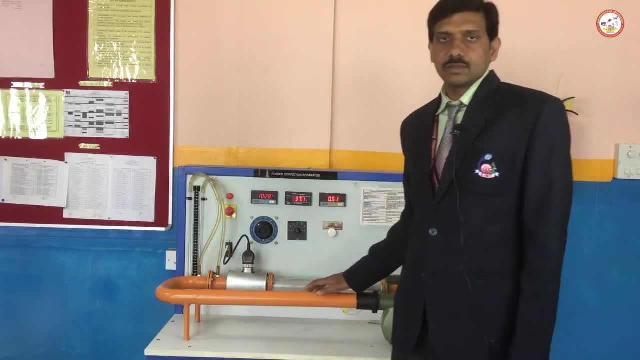 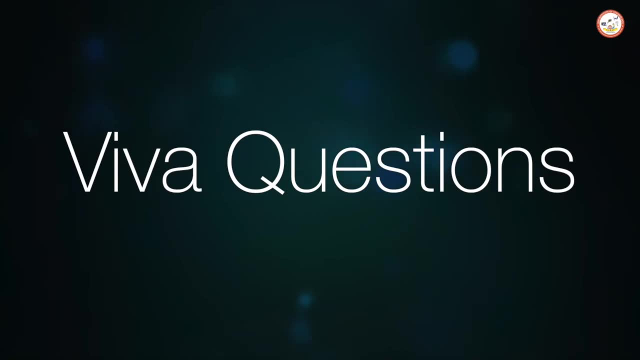 equation. here the H is only the unknown parameters. here There is nothing but the heat transfer coefficient of the specimen. That one you can find out by using that equations. And here you can expect the VIVA question regarding the connective heat transfer. What is the difference? 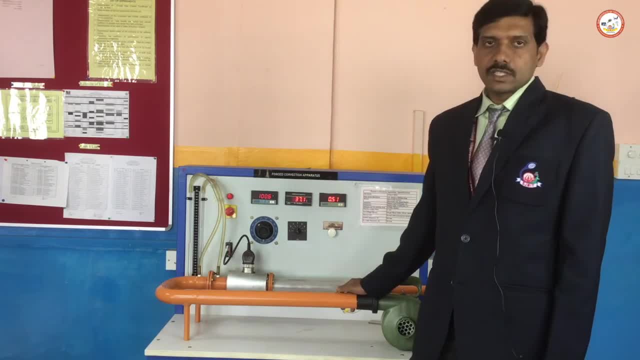 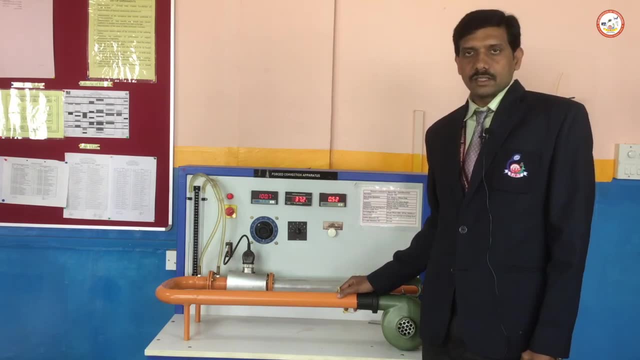 between the natural convection as well as the forced convection And the dimensionless numbers, like the crush-up numbers, nuzzle numbers and so on. So you have to do the calculations. So these are the numbers. And what do I mean by heat transfer coefficient, Like that? you 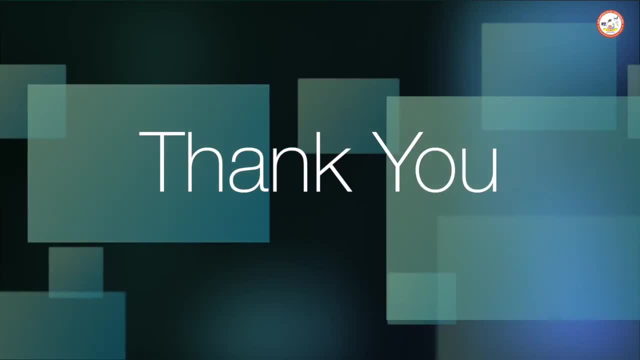 can expect the various VIVA questions in this experiment. Thank you.